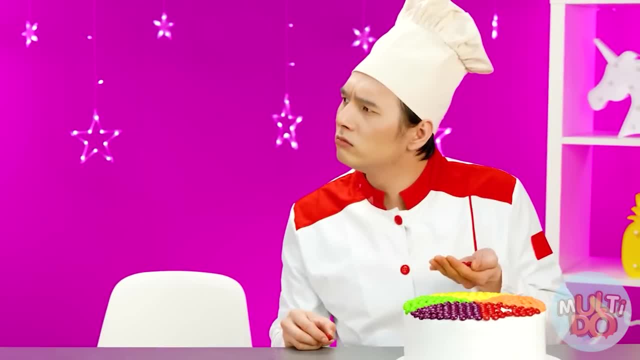 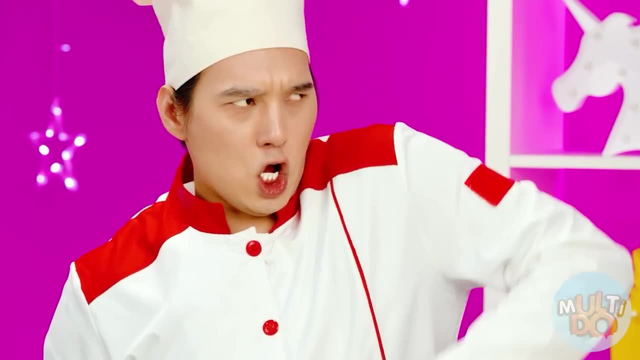 Now you can take a break. Who sleeps while cooking? This is irresponsible. Well, how do you like my cake? Just look at how bright and smooth it is. But it's not all. I want the whole cake to become bright and colorful. 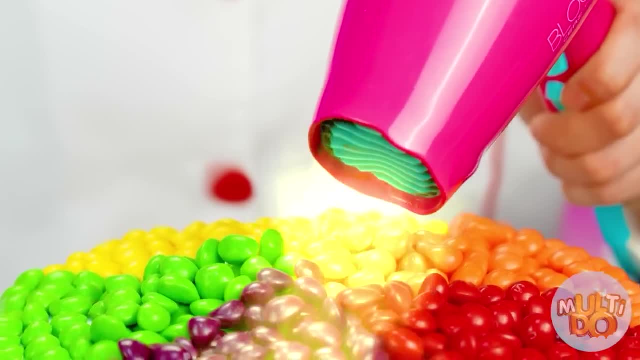 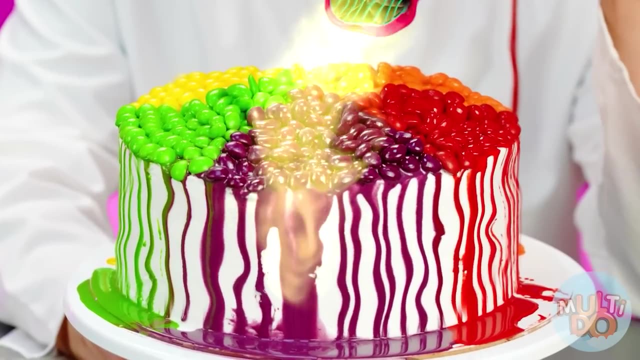 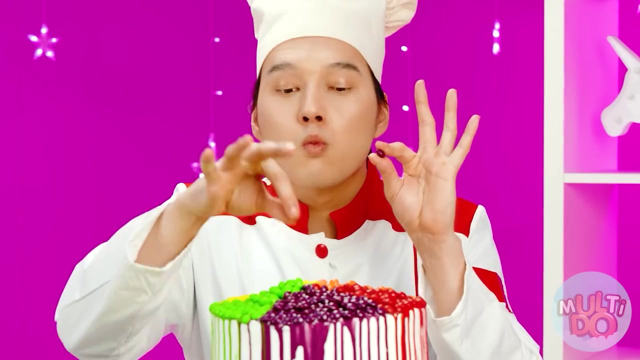 To do this, I need a hair dryer with which I will melt the paint of the Skittles. candies- Perfect. The only thing left is to resort sweets. Bellissimo, Yeah, Just some more here. I think the cake is ready. 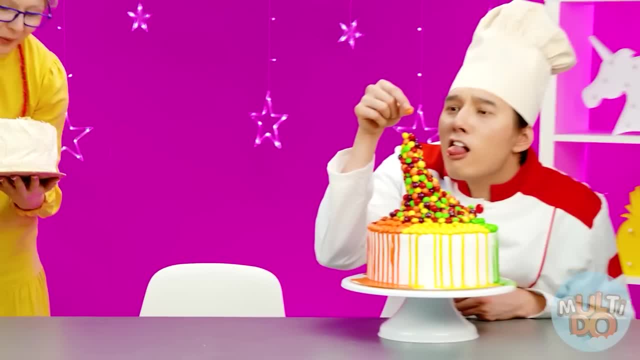 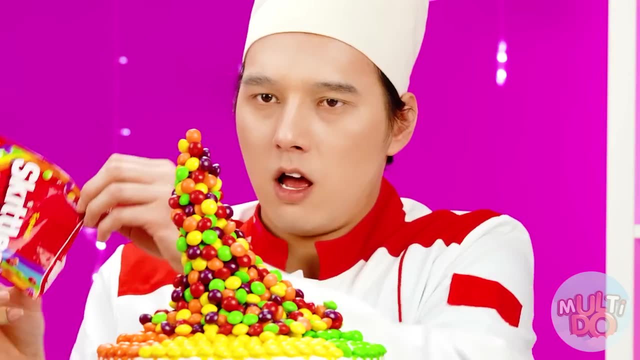 It's time to take it out. I'm sure Betty will definitely like this miracle. I shouldn't have done it for so long. How do you like my sculpture here? I think it's the best thing I've ever done, Oh yeah. 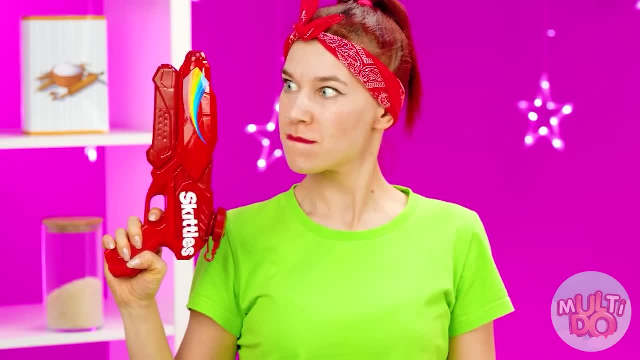 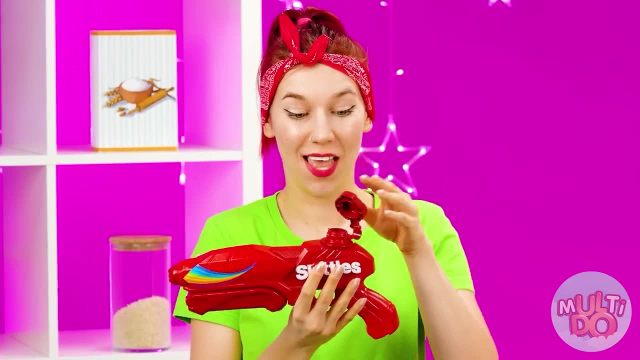 Stop, I also need to cook, Ah. So what am I waiting for? We urgently need to decorate the cake With sweets. To do this, I use Skittles too, But with a gun, Let's do it, Oh no. 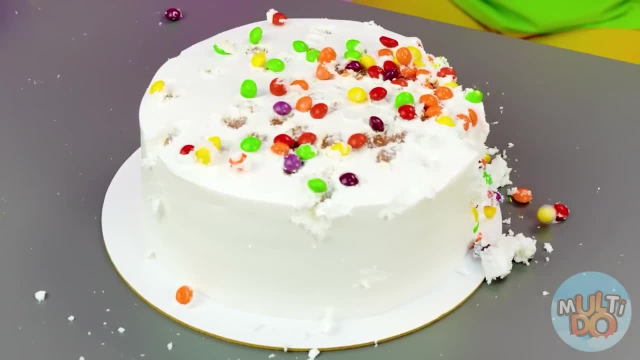 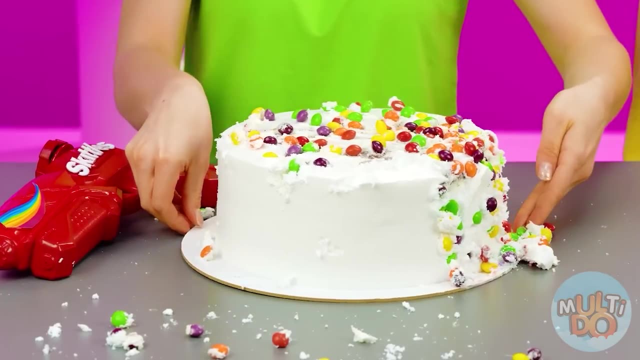 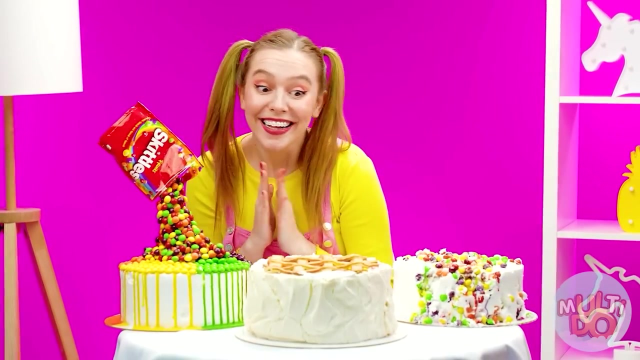 How to… how to manipulate it. Ah, Uh, ta-dam. I think it's ready, Betty. it's time to choose who will be the winner. Bon appetit. All the cakes are very beautiful, Except for the Emma's. 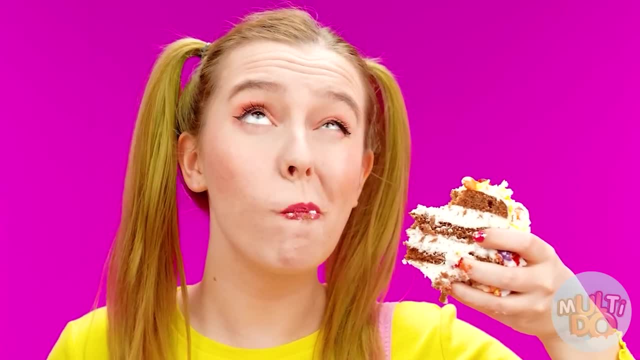 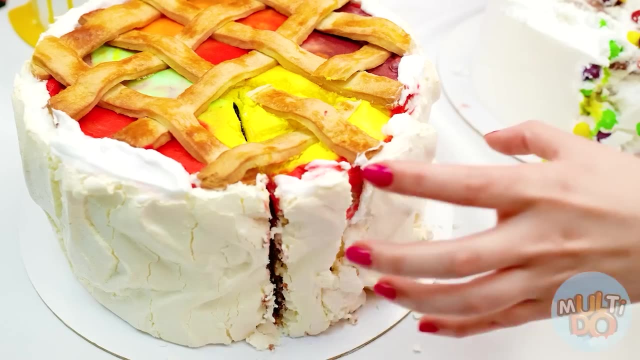 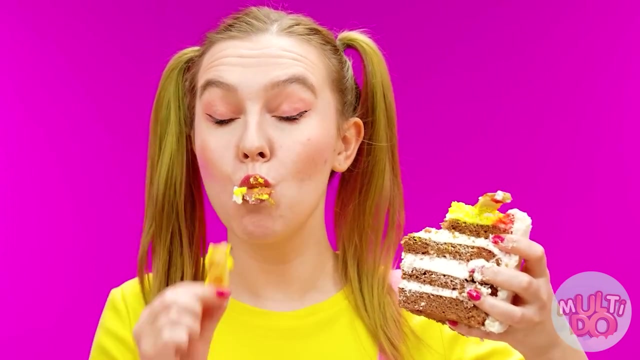 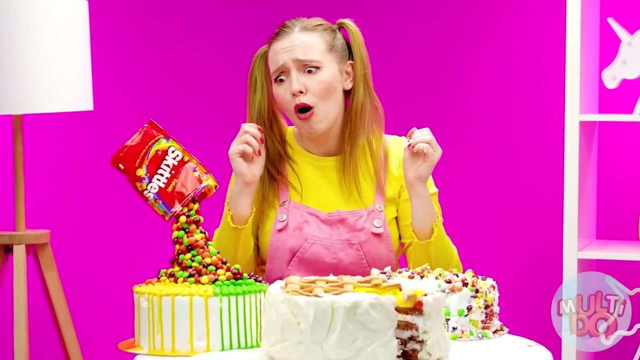 Maybe it means that it's very tasty? Well, no, An ordinary cake. Let's see what awaits me in the middle. Hmm, Well, that's interesting And a completely different matter. Very tasty, Grandma. The one that's left is Chef Zach's cake. 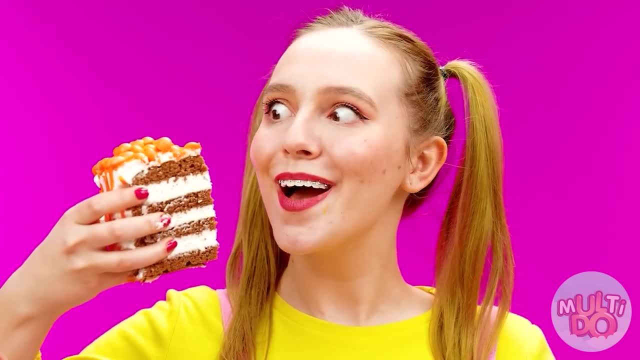 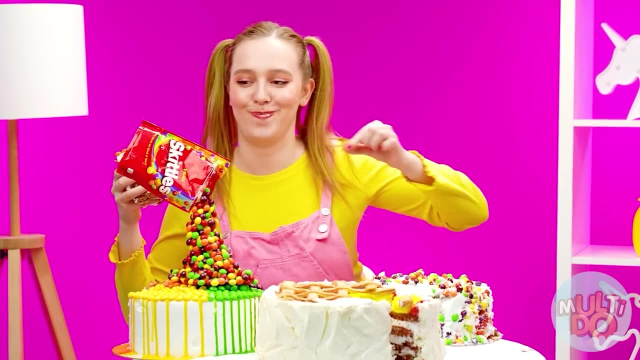 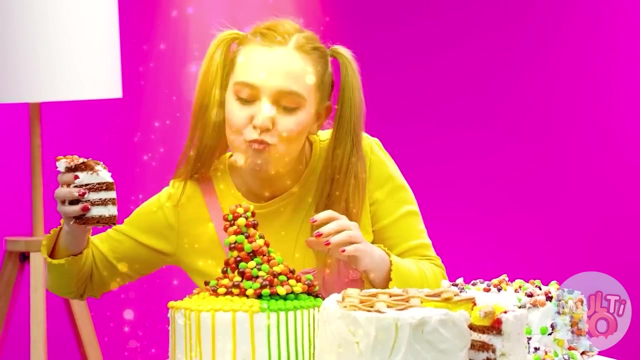 It looks, of course, unrealistically cool. Mmm, it tastes just as cool. I wish I could eat every candy as soon as possible. It's just unrealistically delicious. Zach, you've won. Uh yeah, I knew I was going to win. 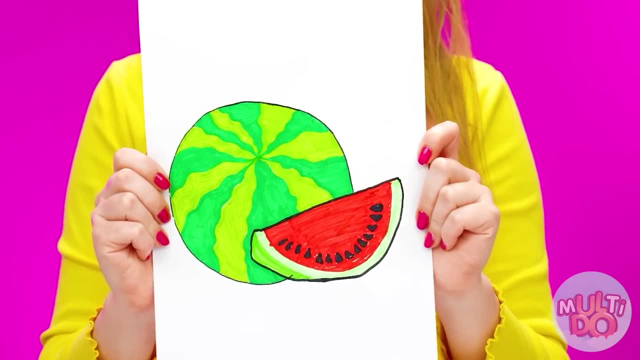 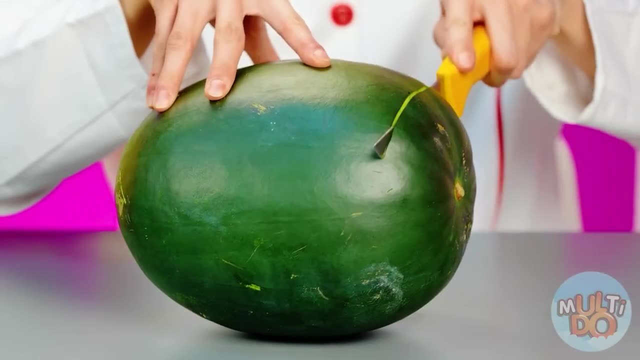 This time I want a watermelon cake. This is a very interesting challenge to my culinary skills. I hope I will come up with a way to make a watermelon cake from a whole watermelon, I know for sure. the first you need to get is to get rid of the excess peel. 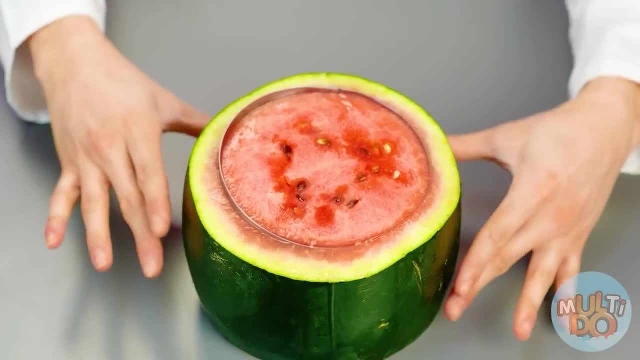 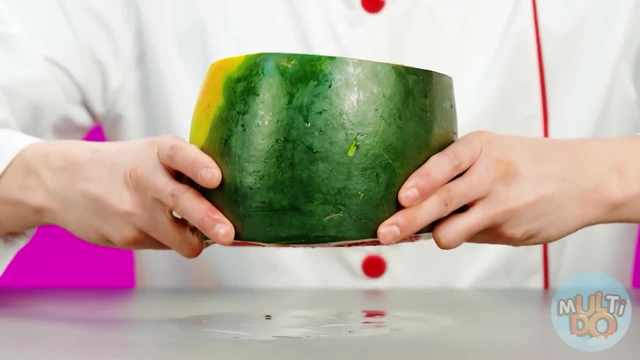 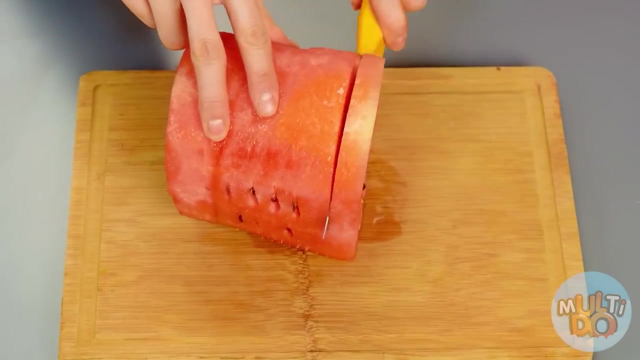 For the cake, I'll use the pulp, Just like this. It's so easy And it will not be a trouble. See, Now you need to cut the watermelon into so-called… cakes. Ugh, I probably won't bother so much. 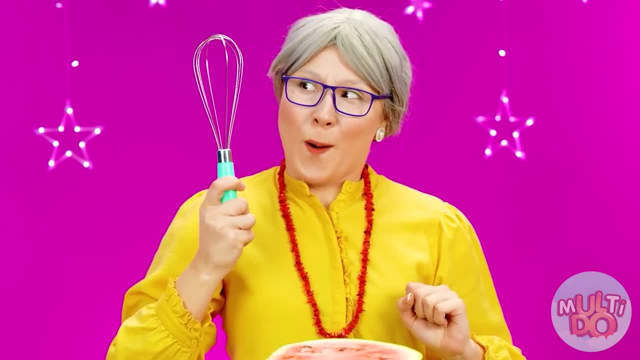 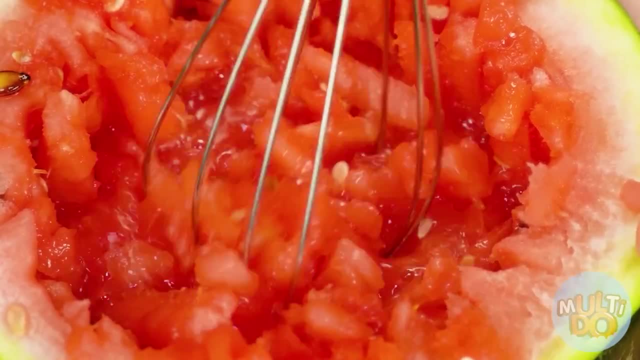 With watermelon, everything is much easier. It's just enough to cut it in half and stir the little gelatine inside. But first we need to put out the pulp And now… Only then you'll add some gelatine. 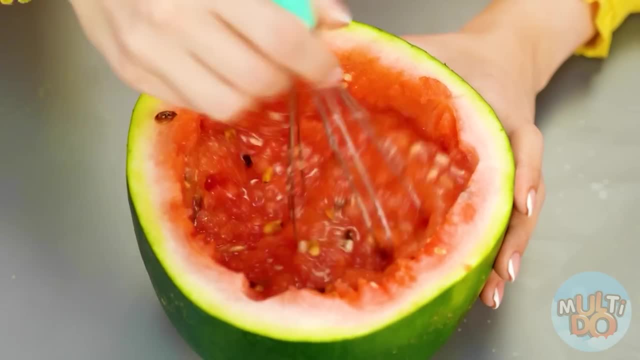 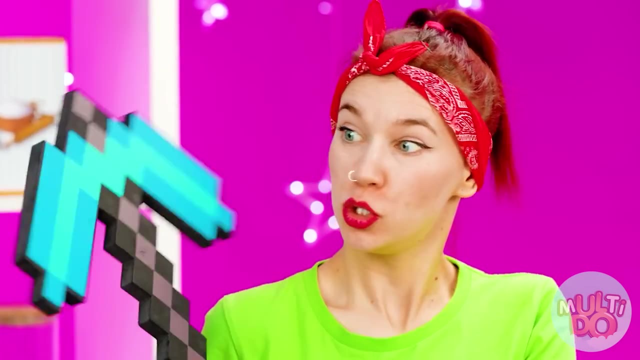 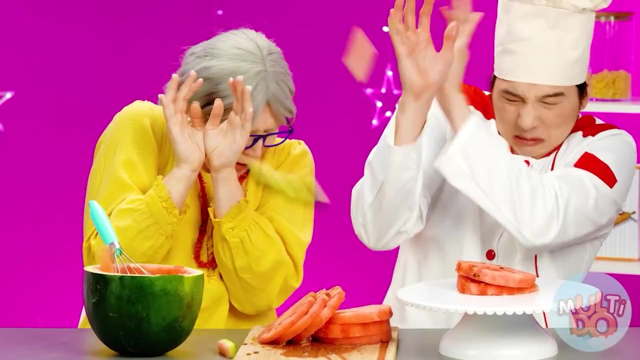 The main thing is to do… Everything very, very carefully. Grandma, It was so cool. Well, I'll smash a watermelon with a diamond pickaxe. Be careful. Uh, stop it. Everything is flying around. Excuse me, I've been playing too much. 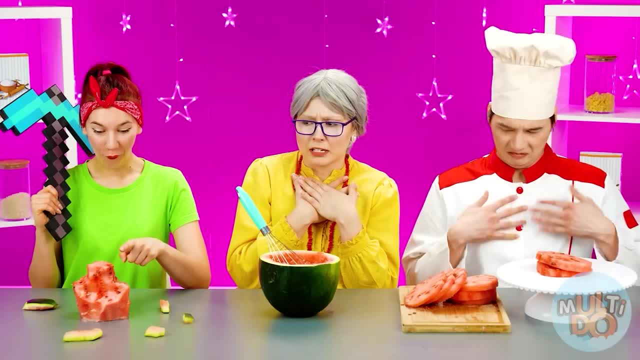 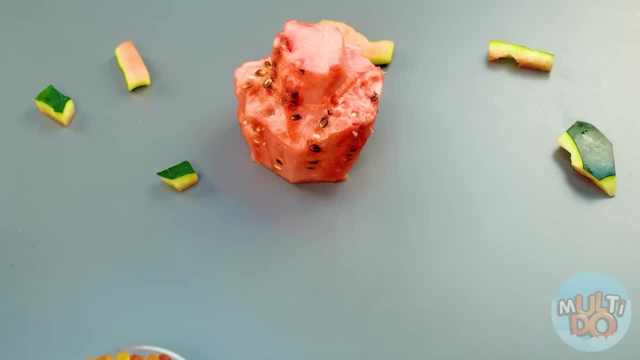 But don't worry, the watermelon's almost finished. Just look at how appetizing this part is. But serving Betty on ordinary… A watermelon is not the case. It'll be much cooler if I decorate a watermelon with various goodies. 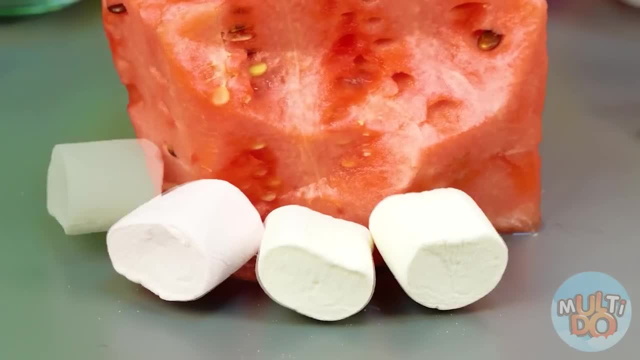 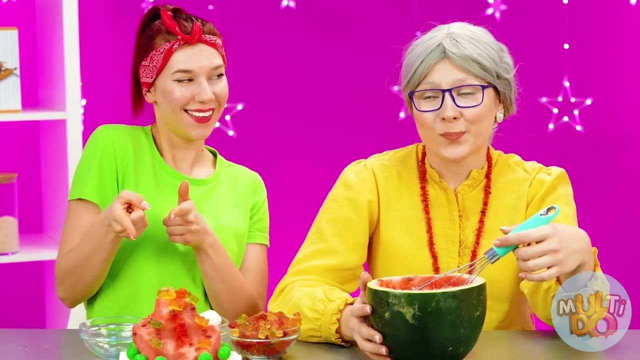 Then it'll be much more like a cake. Just look at it. Marshmallows are so cool And gummy bears Yay. Uh, you call it a cake. That's pathetic. The real cake should consist of several layers. 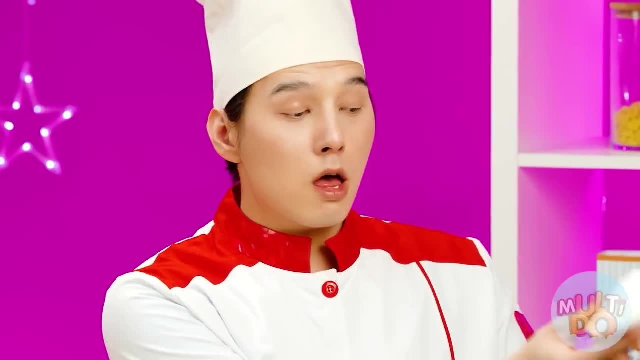 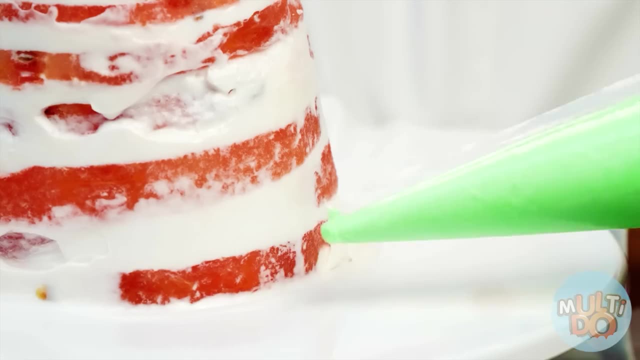 Therefore, it is important to pay attention to this aspect and glue the watermelon slices on. I'm going to start with a special cream. The cream needs to be leveled And it would also be nice to add some color. My cake will be green from the bottom and red on the top. 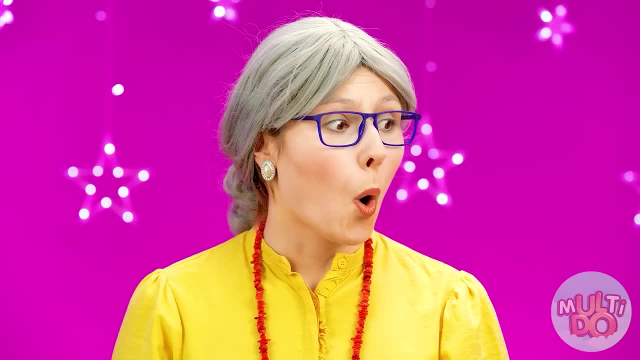 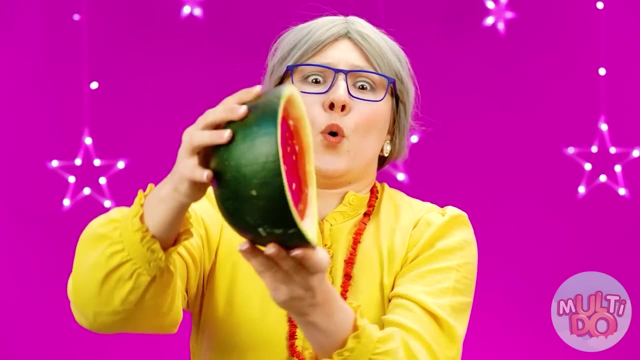 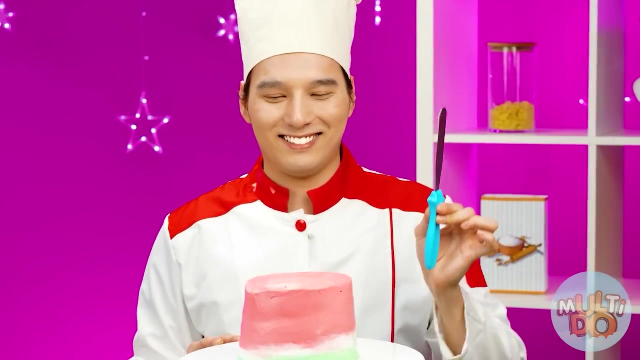 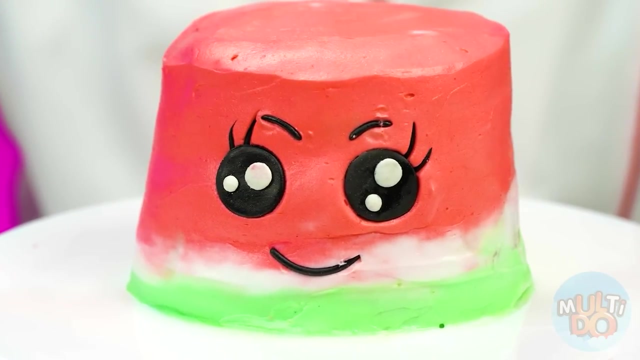 Great color combination for a watermelon cake Doesn't look bad. But I have my watermelon jelly ready, So none of you would have guessed how to cook a watermelon cake. Of course not, because my cake is much tastier. Not only I painted it to look like a real watermelon, I also made eyes. 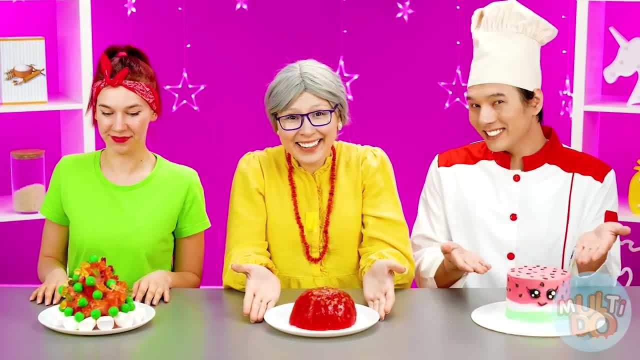 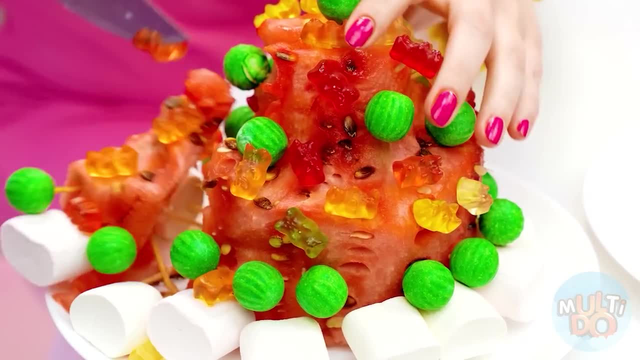 So look how cute it turned out, Betty. it's time to choose which cake you want. Hooray Emma, what did you do? just poking candy into a watermelon? This of course, requires effort, right, And others tried much more. 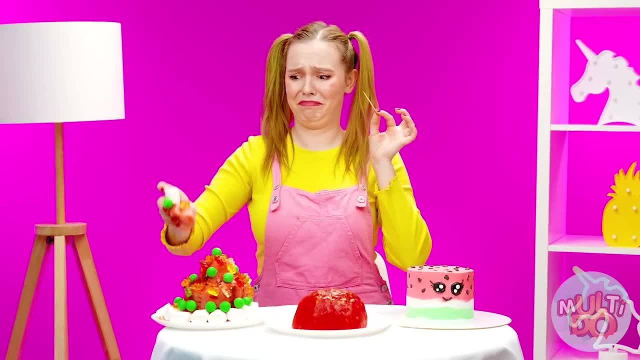 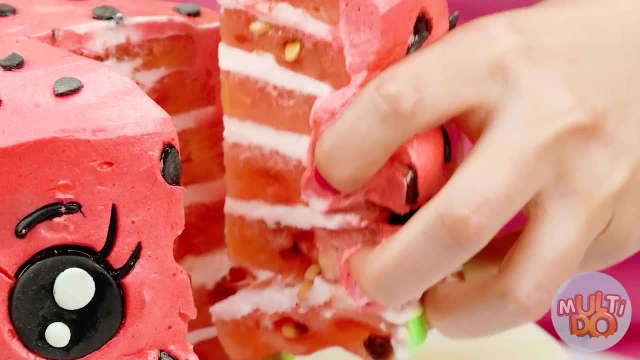 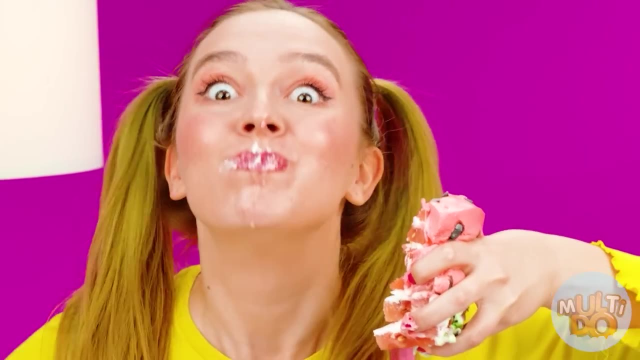 Man, it tastes so-so. I've tasted better ones. Let's see what Chef Zach has prepared for me. Hmm, The cake looks stunning. So good, But is it delicious? Hmm, This cake is simply incredible. The only thing left is to try what my beloved grandma has prepared for me. 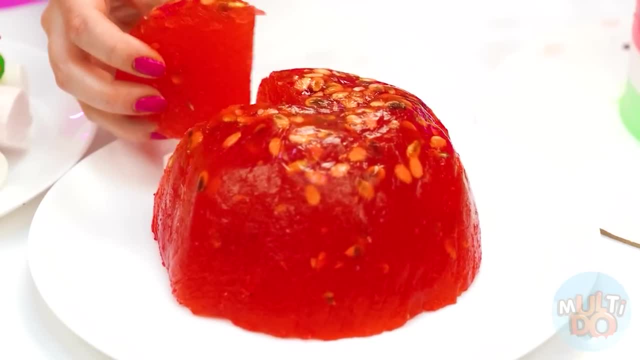 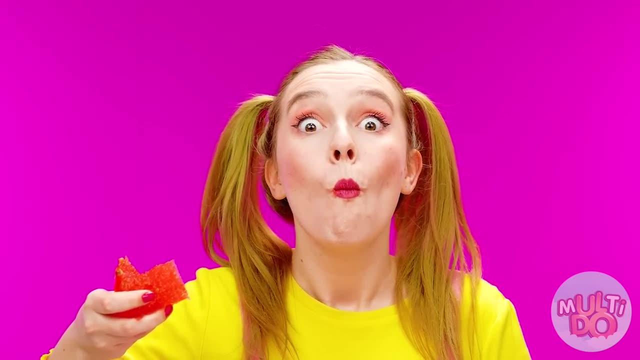 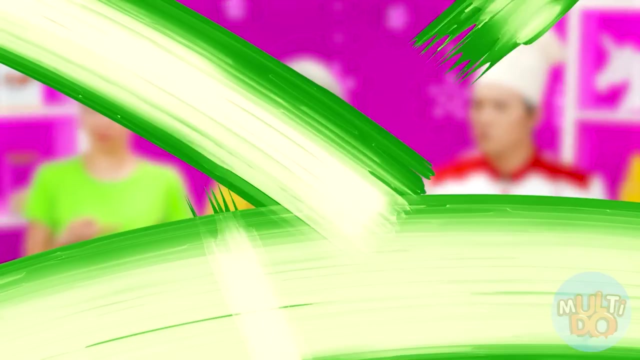 Judging by the texture, I think it's jelly. Hmm, So funny. Yay, grandma, You've outdone everyone today. Ah hooray, I was hoping for it This time. prepare me a cake with a doll. 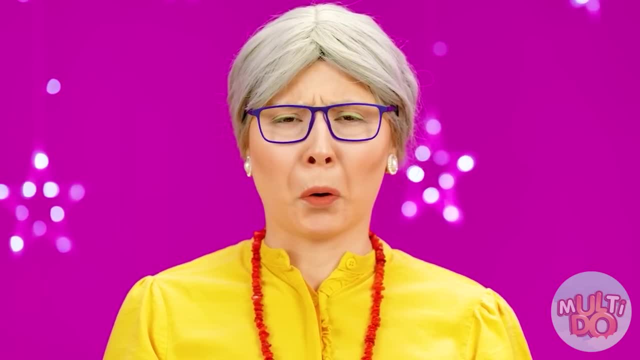 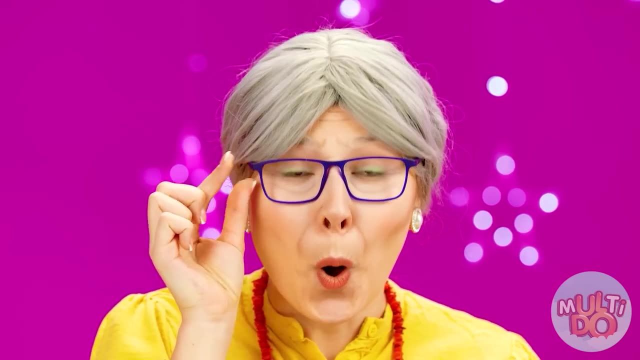 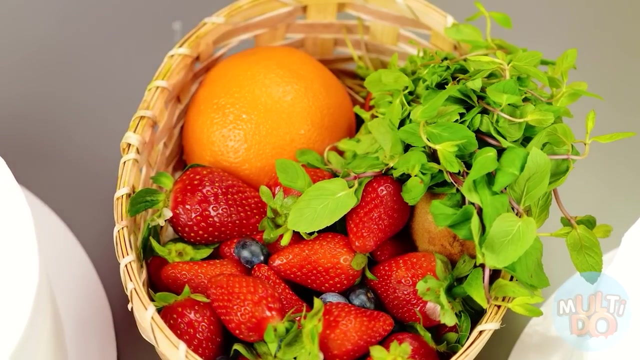 I think it will be an interesting challenge. It's going to be hard. In fact, everything is much simpler, Didn't you see? It's me. I have an idea how to embody you, Betty, right on the cake With these fruits. it'll be very easy. 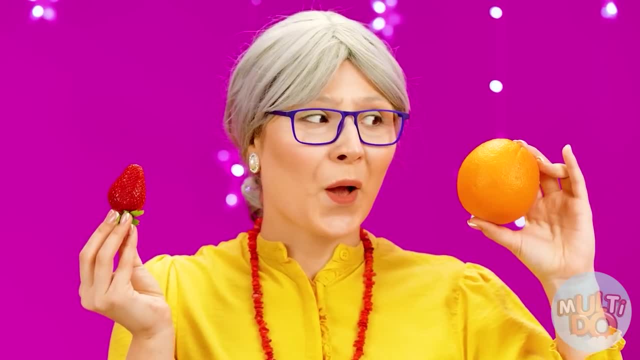 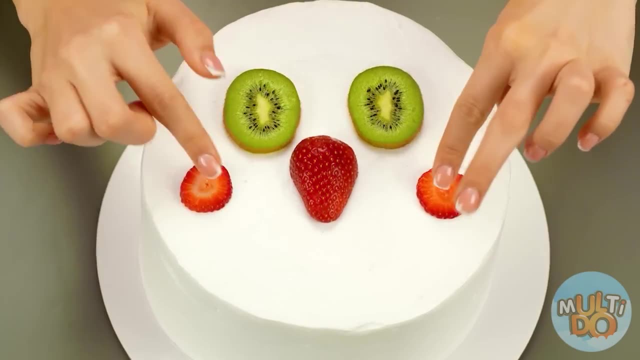 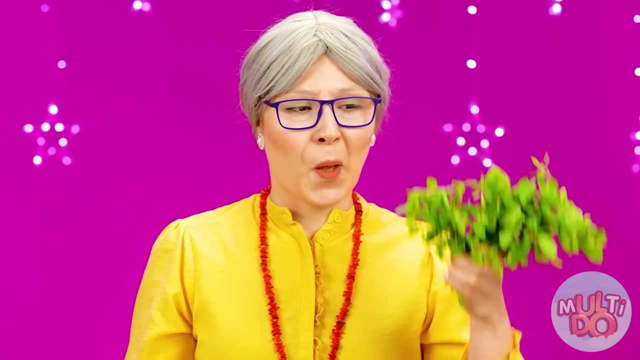 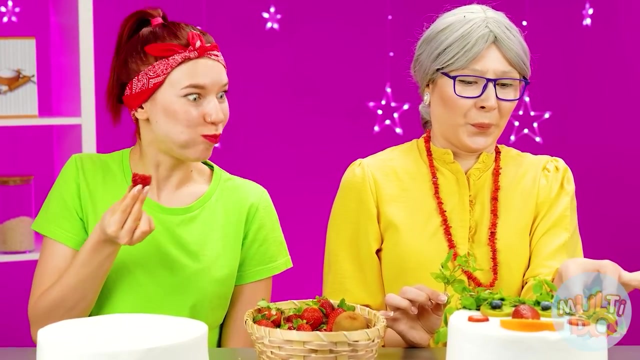 I'll use kiwi And then even more fruits to decorate my beloved granddaughter. Just look at it- So cute. The only thing left is to do the hair And you can serve it. It's a cool idea, but it doesn't look like Betty at all. 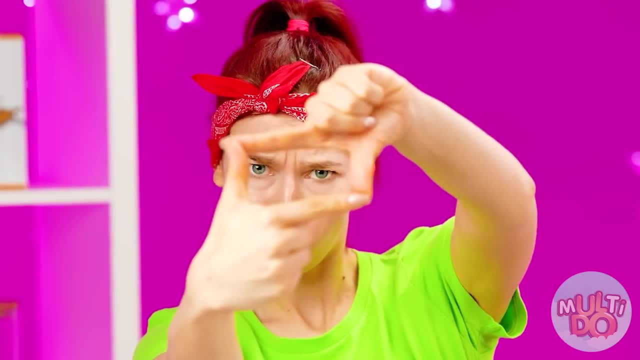 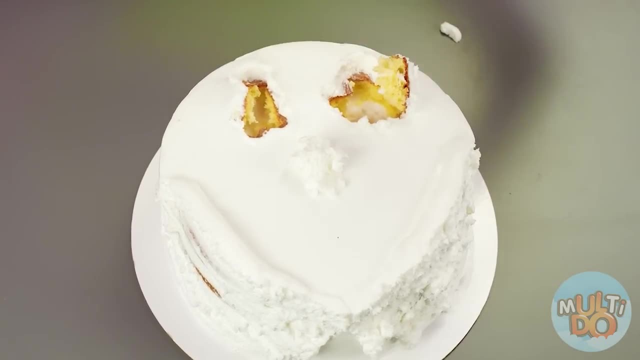 I also love fruits and berries very much. But it's too late to chat. It's time to start working on the cake. To do this, I will first need my hands, Of course. what kind of face without eyes? You need to slap your eyes and eat the cake. 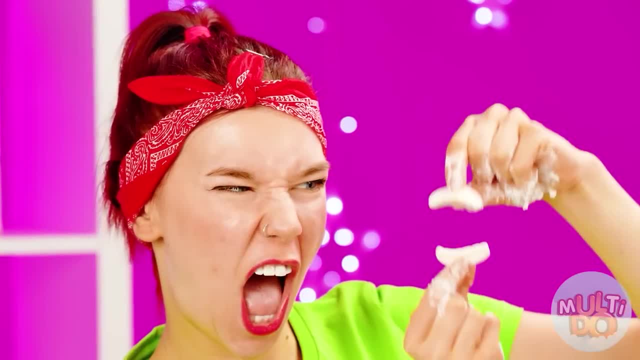 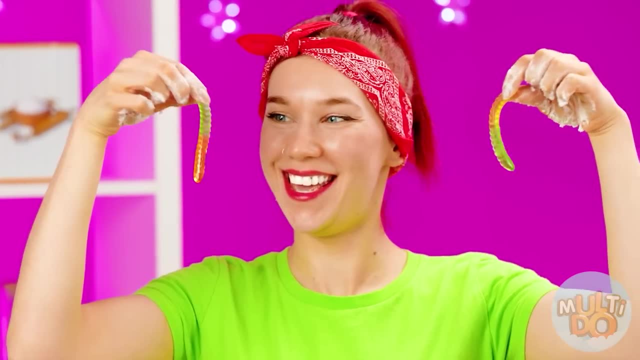 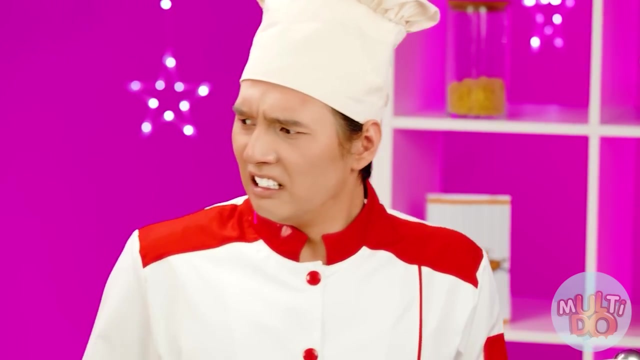 Here are my marmalade eyes, And these ones I'll use to put some mouth on her face. I think it's so adorable. The only thing left is to add some hair and it's ready. Uh, it looks disgusting Like a scarecrow. 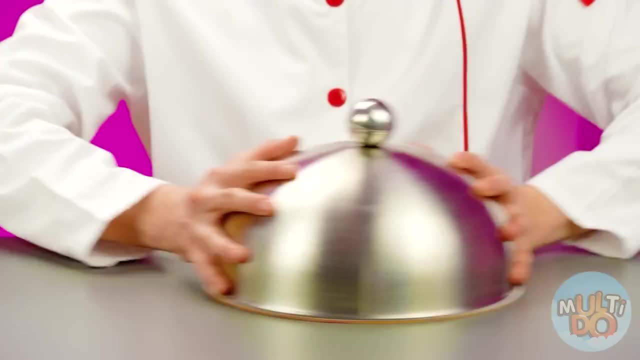 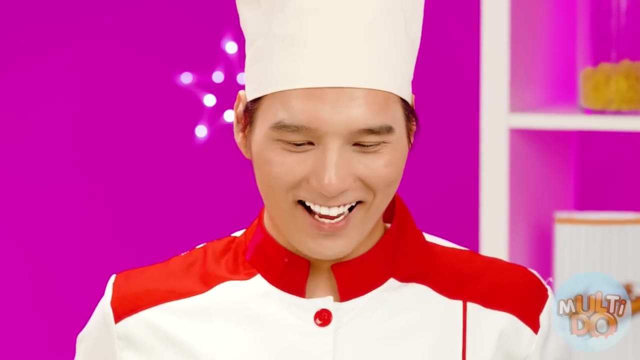 Before I start working, I need to change the shape of the cake and make it round. I dealt with it very quickly. Now I'm going to need a doll that I'm going to put in the cake. The cake will look very pretty. I'll put it in the cake. 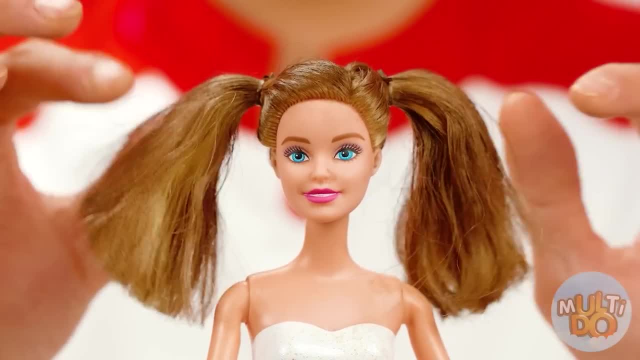 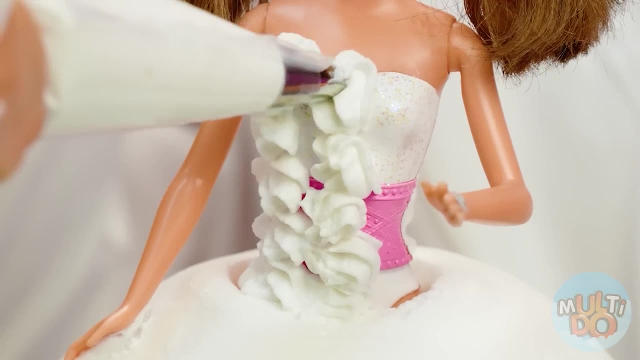 I'm going to put it in the cake. I'm going to put it in the cake. The cake will look very pretty. The cake will look very much like a huge chick dress. Just need to finish it. Of course, cream or whipped cream is perfect for this job. 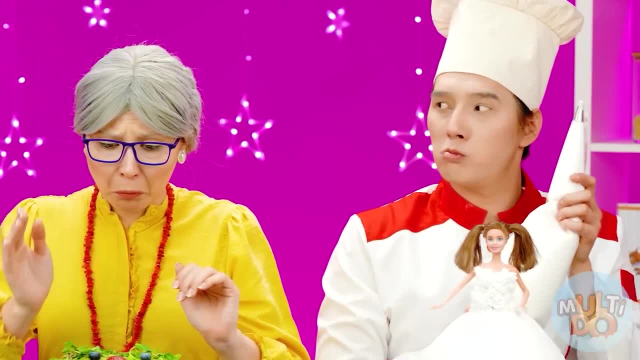 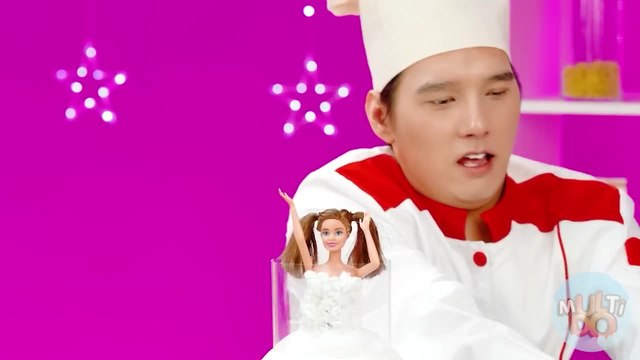 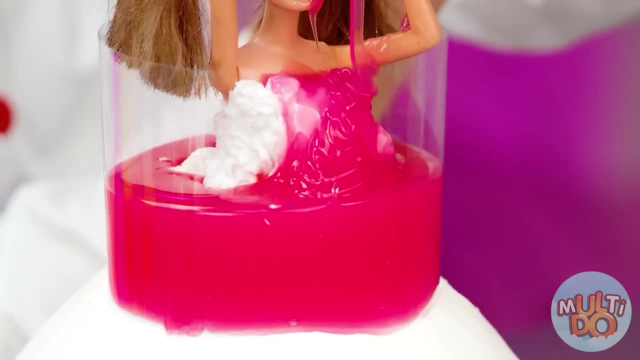 But it's plastic. It's not edible. Uh, stop talking to me, To your cake. So the only thing left is to pour sweet syrup into a special mold, which will make it very beautiful. Oh yeah, Perhaps this is my favorite moment of cooking. 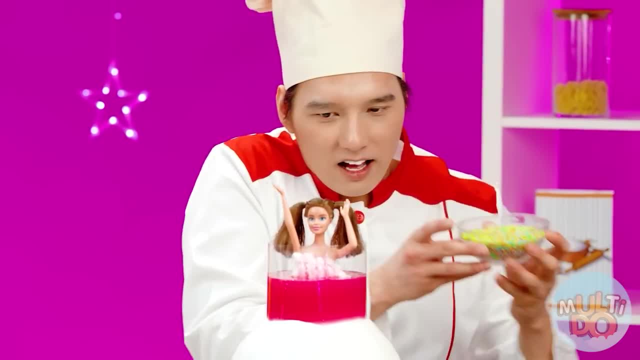 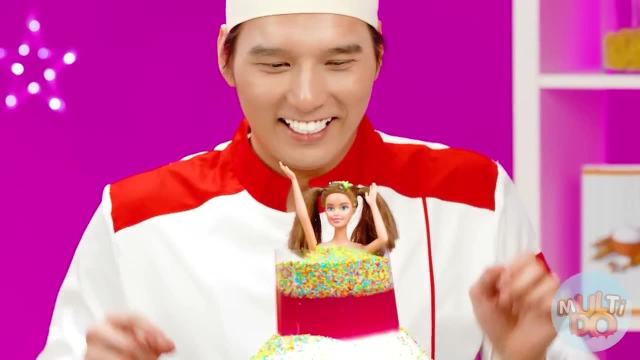 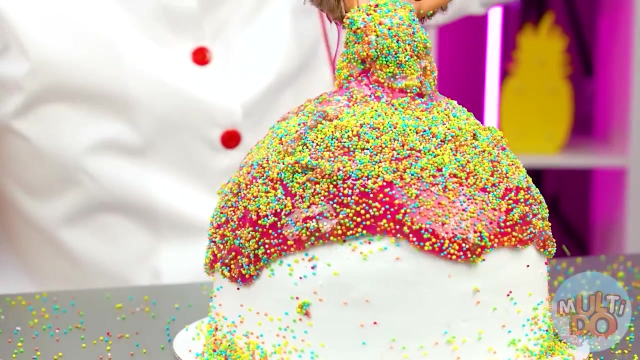 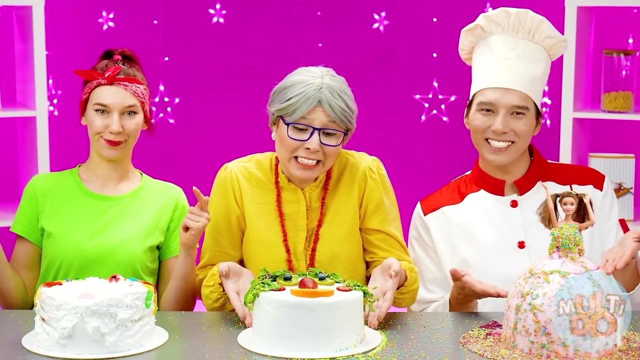 I love it when someone shows off their cake like that. Just some sprinkles, Yeah voila. Well, let's go. I'm sure this dress will be irresistible. Aw, Patty, Have a nice meal. Wow, I'm delighted with every cake. 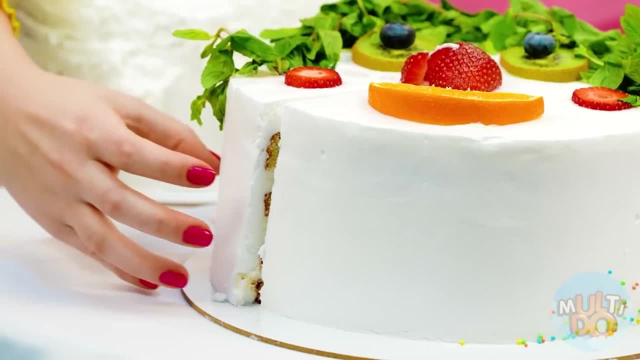 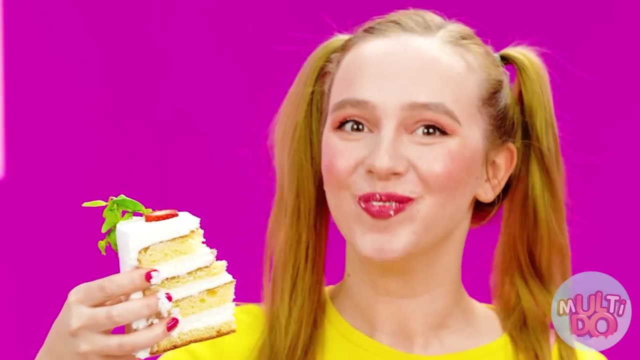 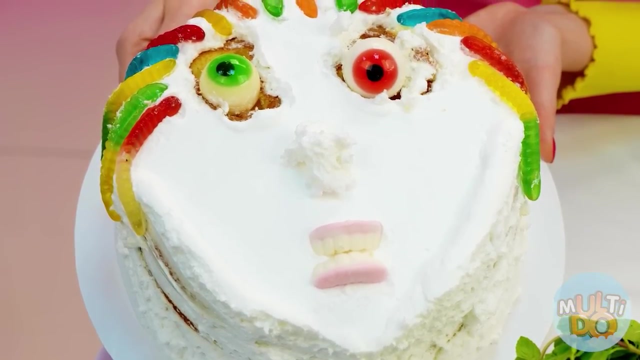 But I'll start with the one from Grandma. Her cake looks unrealistically delicious. Let's see if it's true. Yes, it's so good, But something's missing. Emma, What did you cook? Why does this case have such a scary face? 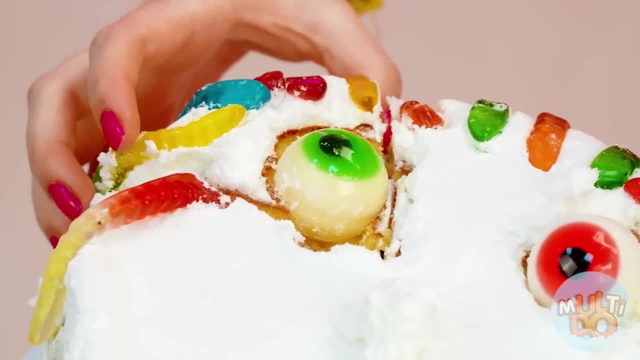 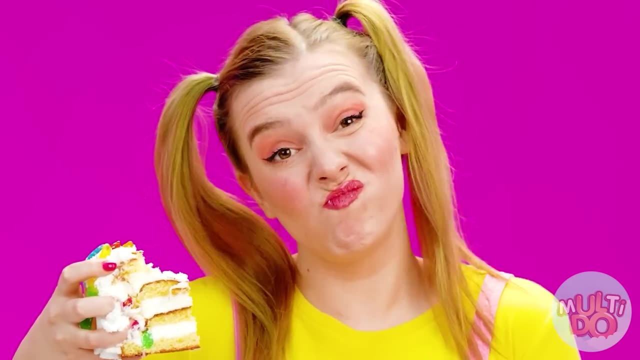 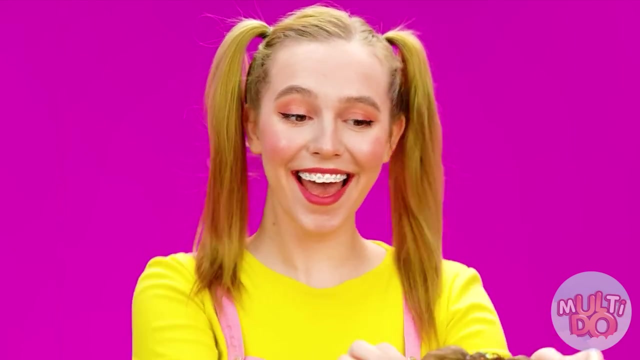 No, it's definitely not like me. I hope this cake is at least delicious. Mmm, usually it's been tastier. Okay, the only thing left is to find what Zach cooked. Wow, it's really the coolest, Because I really look like a doll.